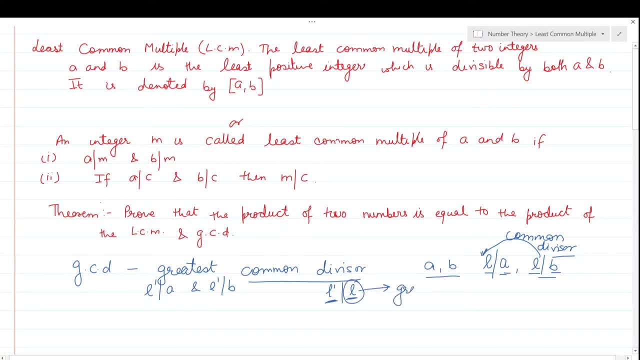 Then we will say that L is greatest common divisor of A and B. So this definition must be clear to everyone. Now, next is: what do you mean by LCM? LCM means least common multiple. This is where the meaning is clear. 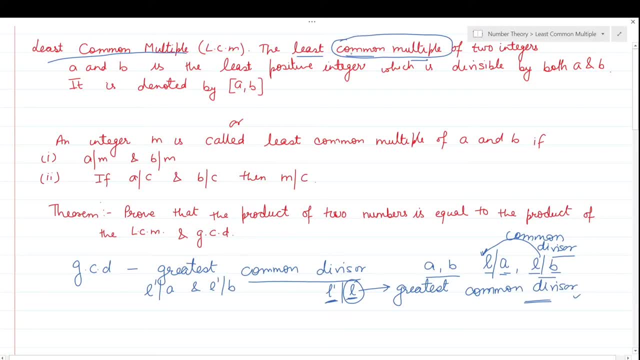 First of all it is a common multiple. Multiple means that which will be divided by both the numbers. Suppose we say that M is least common multiple of A and B, When will M be least common multiple? First it should be a common multiple. 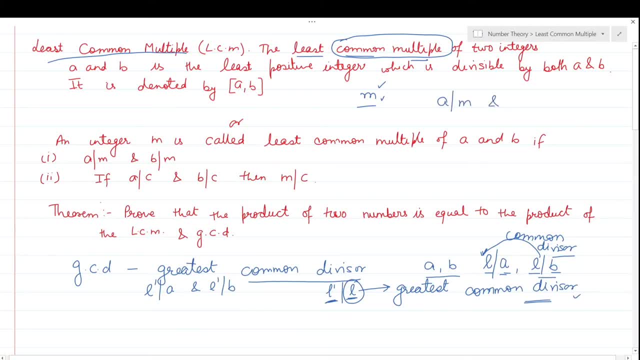 Common multiple means that A also divides M and B also divides M. If we divide A and M, then what do we say? M is multiple of A, And if we divide BM, then we say that M is multiple of B. Now, when we divide both the numbers, 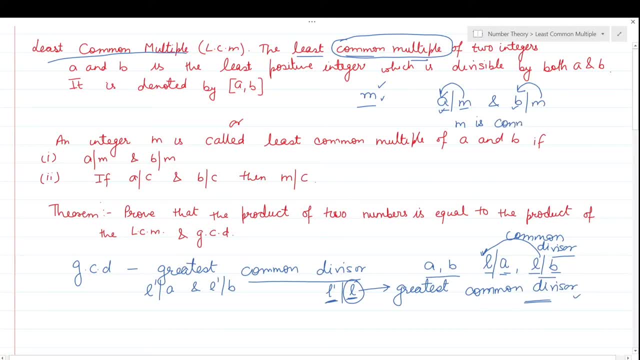 it means that M is common multiple of A and B. Both are multiples. Okay, Now the least common multiple must be a common multiple. Then it should be least. It means it should be the smallest multiple of A and B. Fine, 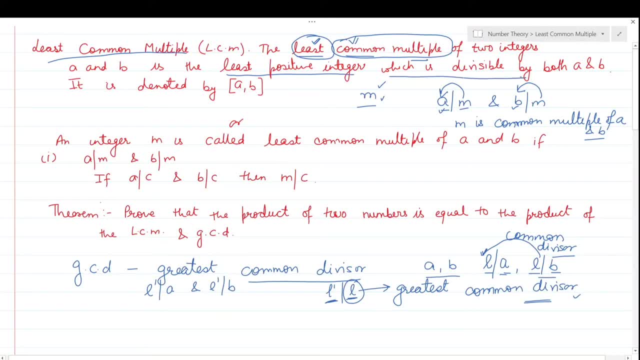 It should be a least positive integer which is divisible by both A and B. If both of these are divisible by A and B, it means it is a multiple of A and B And it should be the smallest integer, like this: Okay, Then M is said to be least common multiple. 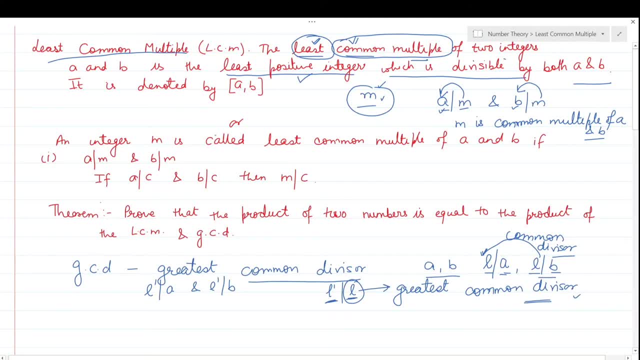 And mathematically, how do we use this? An integer M is called a least common multiple of A and B. if the first condition is that we should divide both A and B, What does this mean? M is common multiple of A and B. 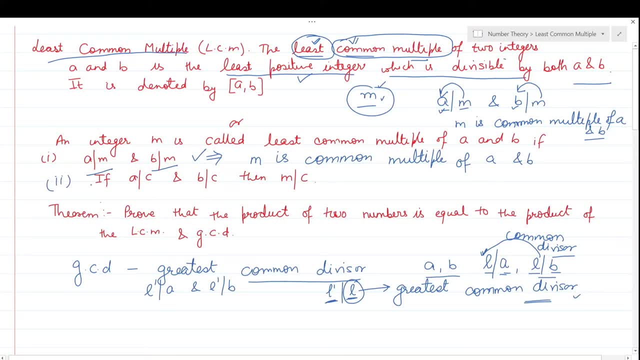 Fine, Now what is the second condition? If there is another number, C, which is divisible by, which is divisible by both A and B, which is the common multiple of both A and B, then M should divide C. Now, M should be the smallest among all these common multiples. 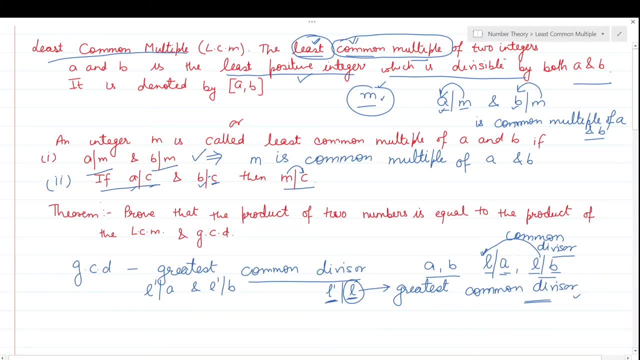 When will it be the smallest? When it will divide all those common multiples? Okay, So this means what is the meaning of least common multiple, Which is common multiple of both the numbers And if there exists any other common multiple? 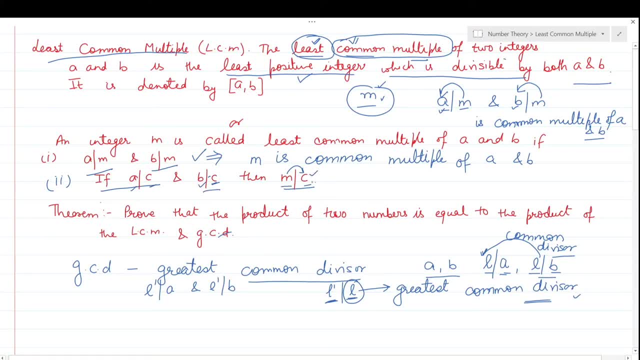 then M should divide that number, that common multiple. Then what will it become? Least, the smallest. It should be least among all the common multiples. To make a common multiple, it should be divisible by both the numbers. Then to make it least, 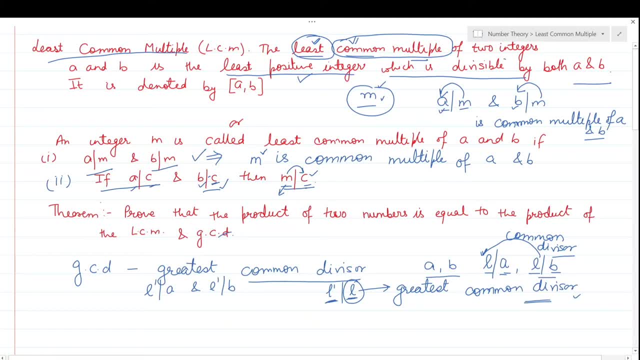 if there are any other multiples, then all those multiples. what should M do? Divide, Fine. Then we say that the least common multiple of A and B Clear Now. next, we are going to prove this result. 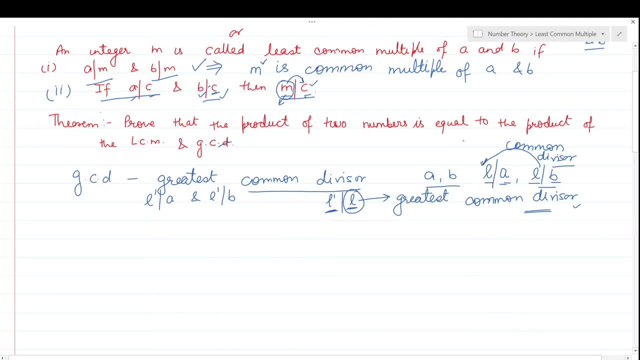 Prove that the product of two numbers is equal to product of the LCM and GCD. Fine, Now what do we have to prove? If you have two numbers, A and B, then their product is equal to product of their LCM and GCD. 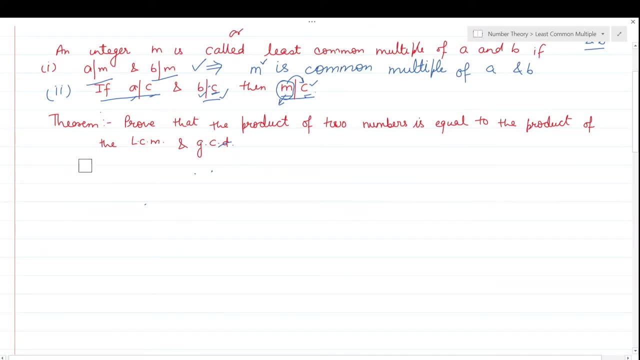 Okay, How will you prove it? Let A and B are any two numbers, We represent LCM with this symbol. If this notation is written, it means it is LCM of A and B, And if you are writing this, it means GCD of A and B. 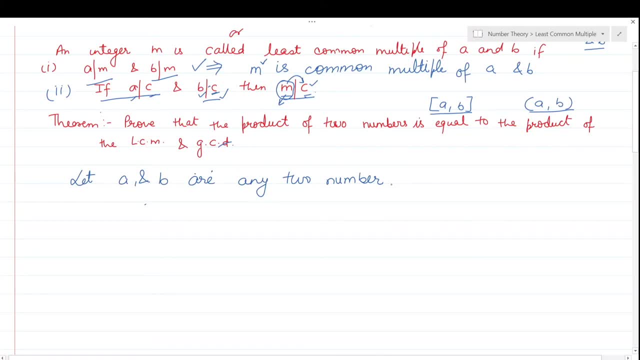 Right Now, let A and B are two numbers And LCM of A and B is supposed to be L And GCD of A and B is supposed to be D. Now first let us find out the value of this L. 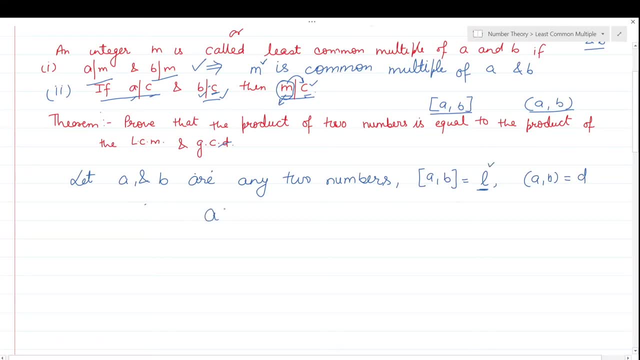 Let us find out the proof that we have to prove. How will we prove it? What you have to prove: Product of the numbers is equal to product of their LCM and GCD. Okay Now, first of all, if the GCD of A and B is D, 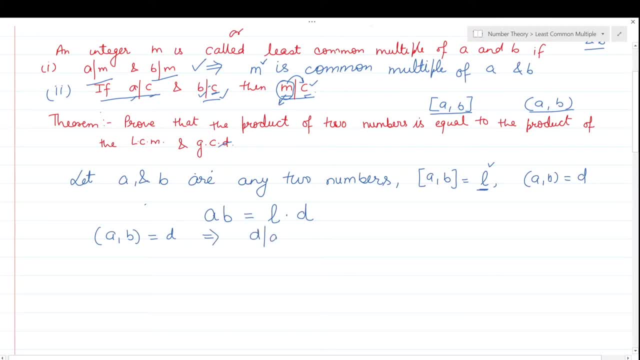 what does this mean? D divides A And D also divides B. If D divides A, then how will A be written D into some Q1.. And D divides B? How will B be written D into some Q2.. 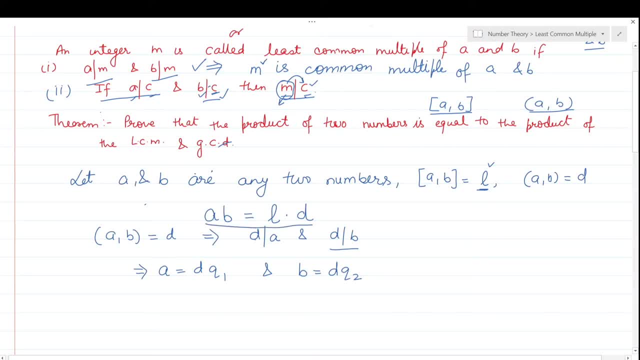 Right Now. if I substitute these values here, what will I get? It is D times Q1 into D times Q2 is equal to L into D. Now, from here, D cancels out. So what do you get? 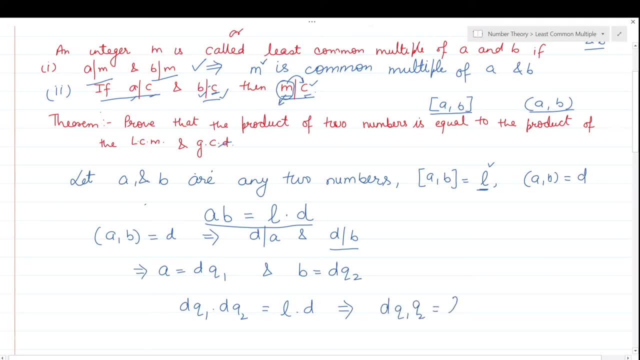 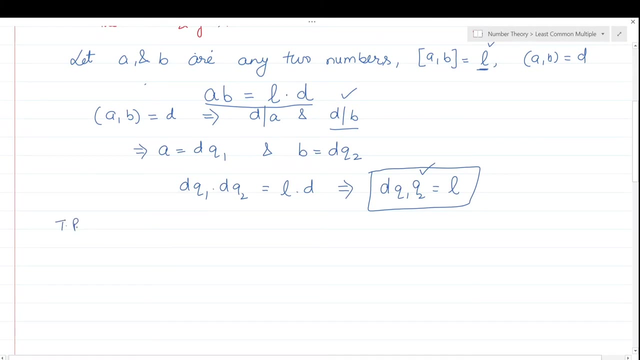 D times Q1, Q2 must be equal to L. So to prove this result we have to prove the LCM of A and B is equal to this value: D times Q1 into D times into Q2.. Okay, Now to prove. 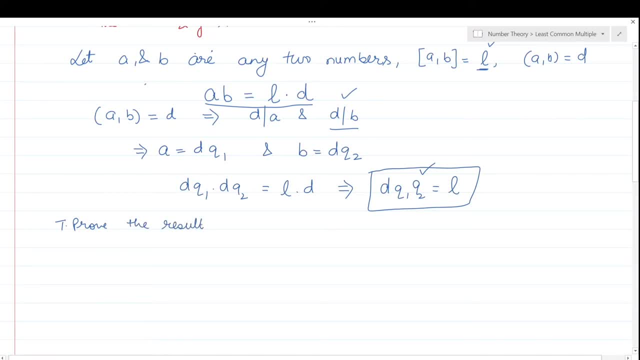 the result. what is the result? AB is equal to LD. We have to prove that D times Q1, Q2 is LCM of A and B. Now, when will this LCM be? First thing, it should be a common multiple of A and B. 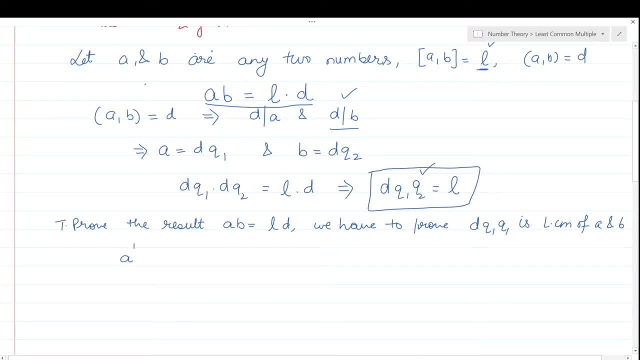 It means A should divide this Before common multiple. this should be a multiple Right. This means we have to prove that AB divides this and B also divides this. Is it true or not? What is A? What did we mean by A? 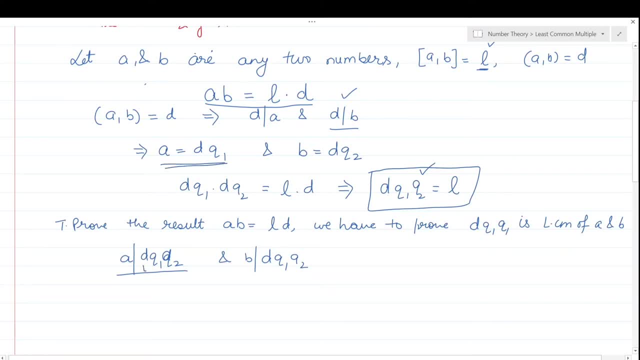 A is D times Q1.. It is what D times Q1 into Q2.. So this number is nothing but multiple of D times Q1.. And A is D times Q1 only. It means obviously, what does A do? 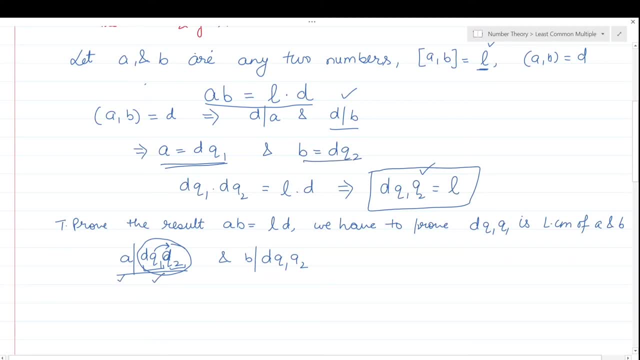 It divides Now what was B. B is D times Q2.. And here what is this? D into Q2, into Q1.. So it is again a multiple of DQ2.. It means B also divides this number. 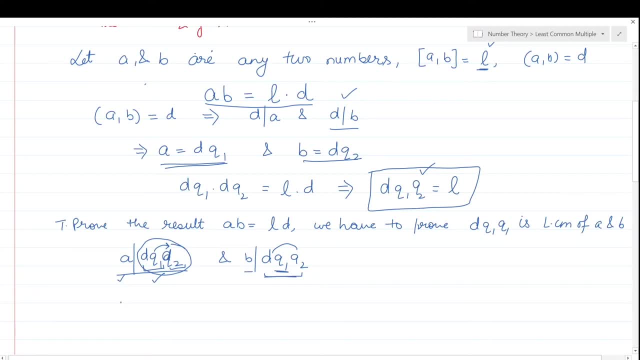 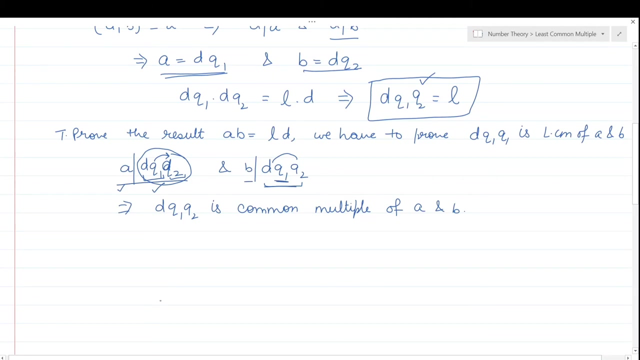 A also divides this, B also divides this. This implies that D times Q1 into Q2 is common multiple of A and B. What happened to these two numbers? Common multiple Now? what do we have to show? It is not only a common multiple. 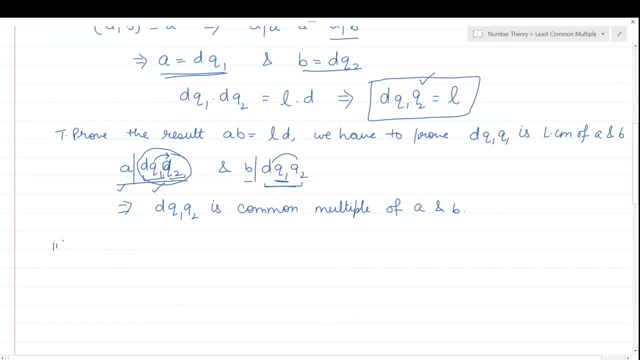 It is a least common multiple. So what do we have to prove for least common multiple? If A divides some number and B also divides some number, It means, if there exists any other common multiple, then what will be the least common multiple of this number? 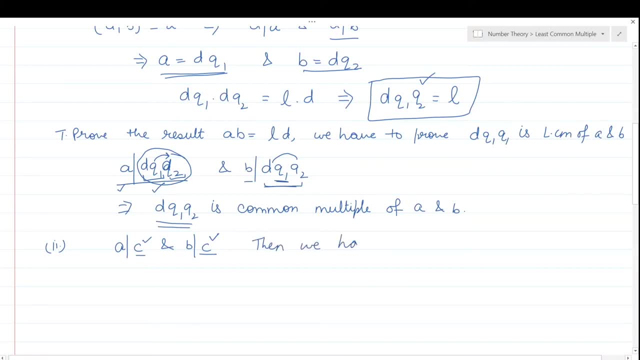 Then we have to prove. Then we have to prove: D times Q1 into Q2 divides this. If this is divided, then what will be this Least common multiple? Now you have given that A divides C, So I can write C as: 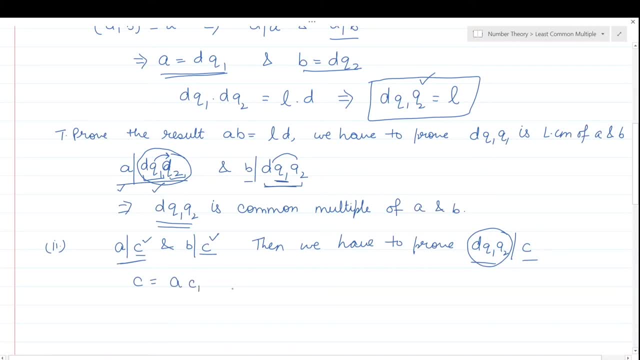 A into some C1. And B divides C Means we can further write C as B into some C2.. Okay, Now C is the same. It means AC1 is equals to BC2.. Clear, Now we will put the value of A. 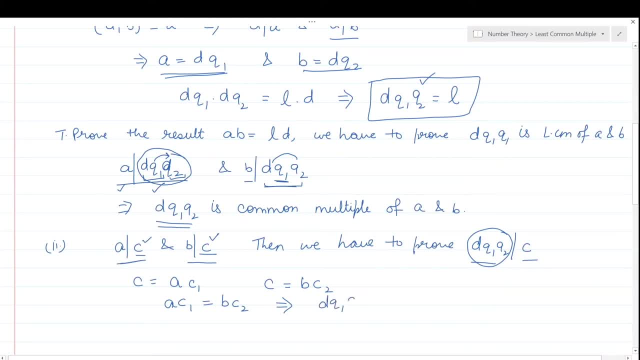 What is the value of A? That is equals to D times Q1 into C1.. And what is B? D times Q2 into C2.. We have substituted the value of B and A from here Now. D cancels out. 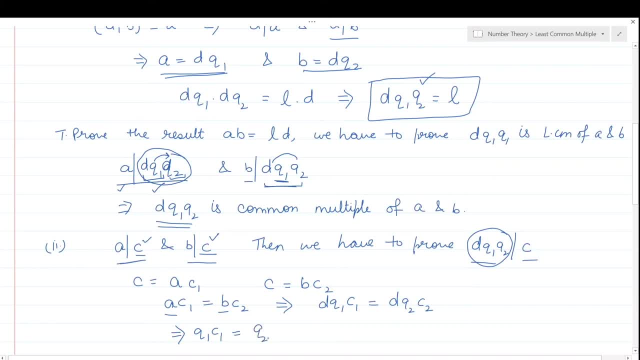 It means Q1 times C1 is equals to Q2 times C2.. Yesterday we had done a result If out of two numbers, their maximum common part, greatest common divisor. if we take out the common part, then the remaining terms. 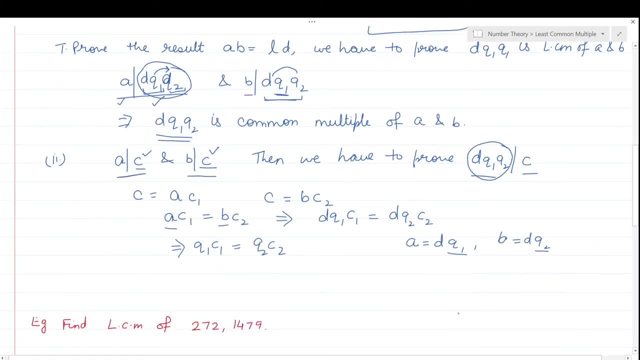 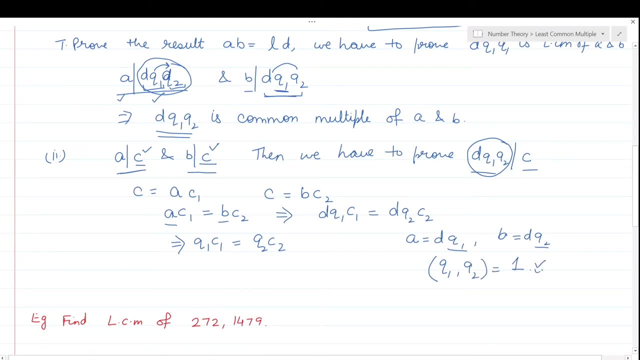 that is, A by D and B by T, which is here, is equal to Q1 and Q2.. So between the remaining two numbers, the GCD is always 1.. Okay, Now we are going to use this result. 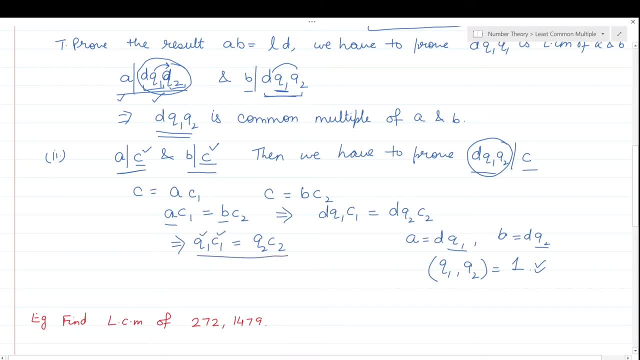 Now what did we get here? Q1 into C1 is equals to Q2 into C2.. This means this number is a multiple of Q1. Because Q1 into something is written, This means Q1 divides Q2 into C2.. 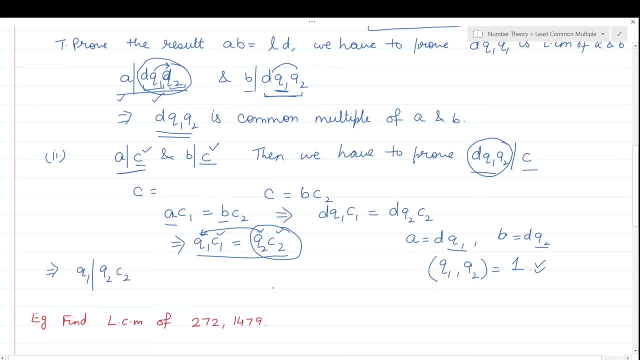 Now you had done one more result. If one number, if A, divides product of two numbers and GCD of this number with one of them is 1, then it divides the second one. What is here? Q1 divides Q2 into C2.. 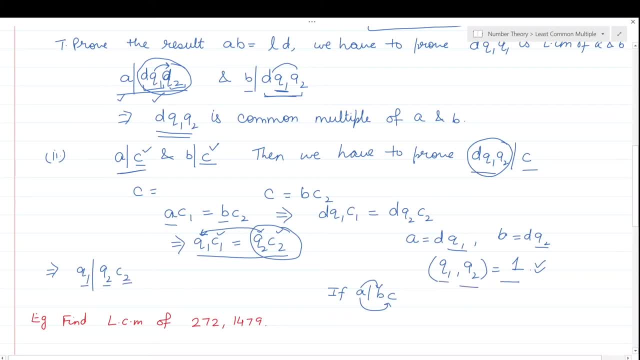 And Q1 and Q2's GCD is 1.. So it means that result tells you that Q1 divides C2.. Okay, Now Q1 will divide C2.. If Q1 is dividing C2,, then 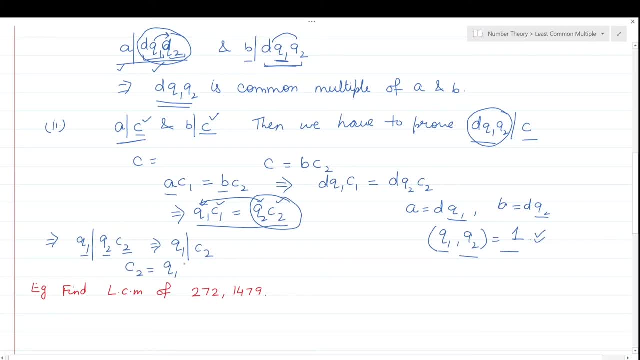 what can we write? C2 is equals to Q1 into some T Did you write its multiple? Okay, Now let's substitute the value of C2.. C is equals to what did we have A times B, times C2.. 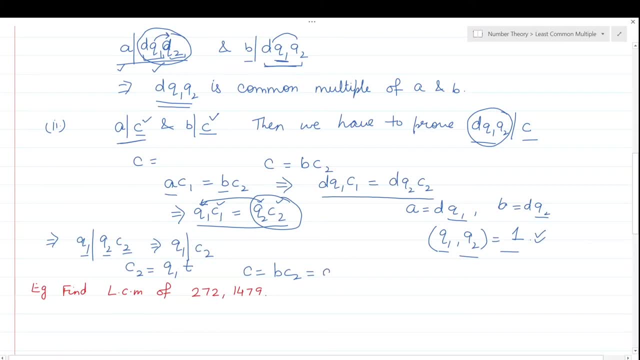 Here. let's put the value of C2.. So what will come? Put the value of B also. So this is D times Q2 and C2 is Q1 times T. So this means this into something is equals to C. 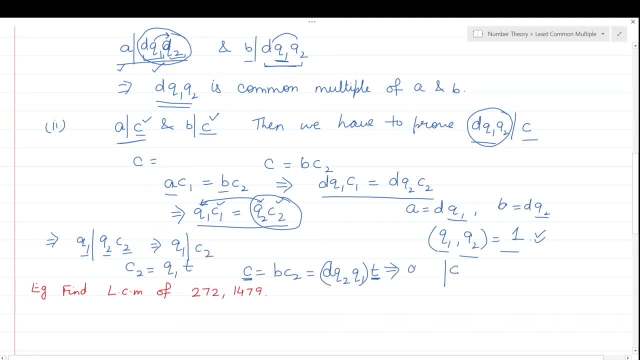 So what it means? C is divisible by what is? it divided by D Q1 Q2, And you had to prove that D Q1 Q2 divides C. So what does this mean? This implies that D times Q1 Q2. 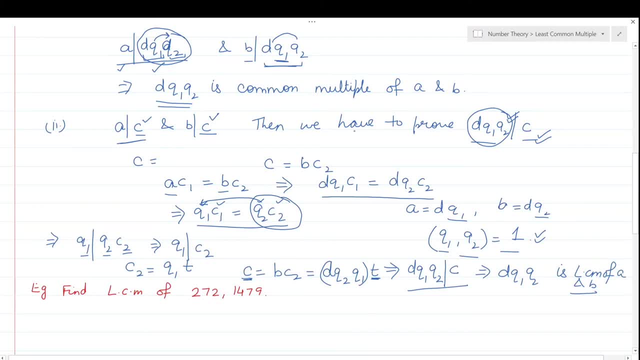 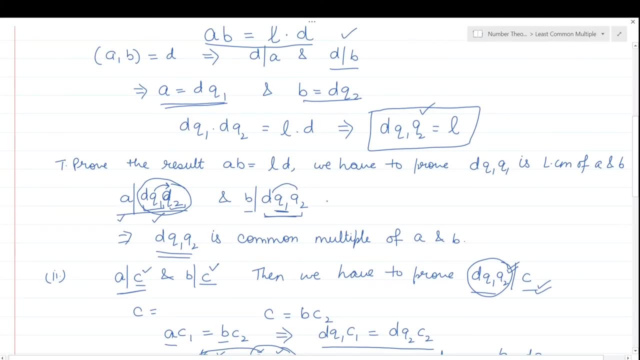 is A and B Right, And if this is LCM of A and B, then what will be proved from there? What we had to prove Right, The result we had to prove. we had brought it here. What we had to prove. 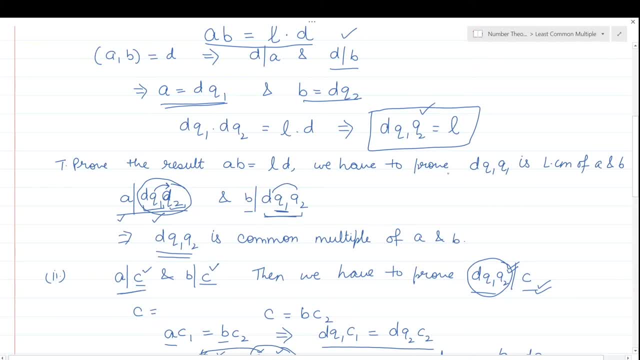 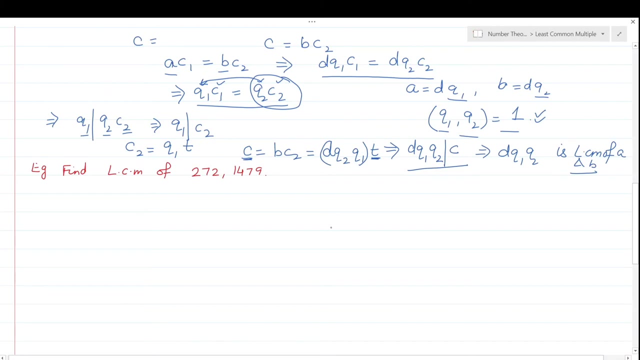 A into B is equals to L into D. And to prove this, what did we make? We have to prove D times Q1. Q2 is LCM of A and B, So the product of any two numbers is always equal to their LCM. 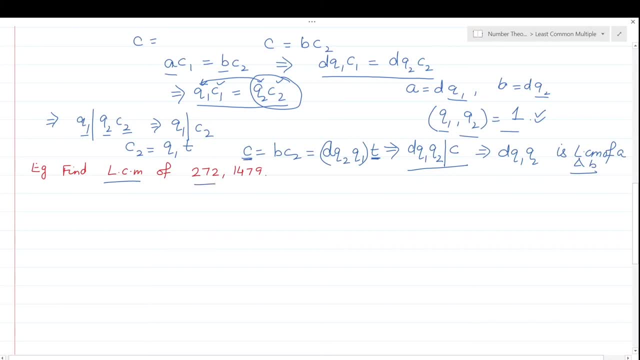 and the product of GCD. Now we have to find out LCM of these two numbers. We will prove this by using the result above. So first we need the GCD of these two numbers. What did we do to get GCD? 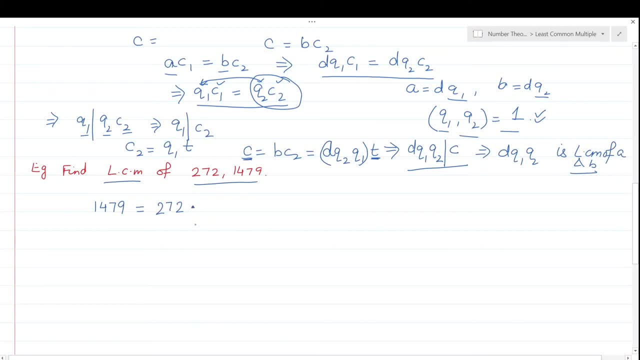 We divided a bigger number by smaller number, Right? So if I divide these two numbers, then what will you get? We will divide these two numbers by 272.. I think the maximum will go from 5 to 6.. So 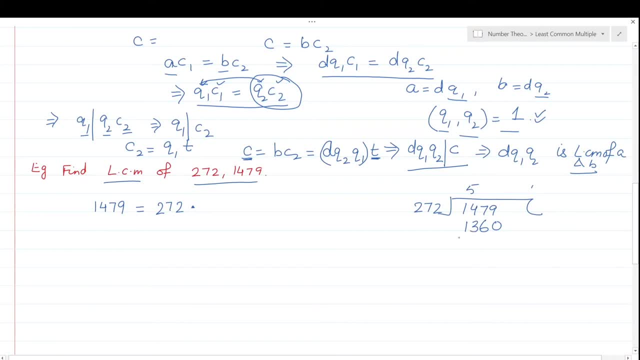 let's check: 5 to 10. 1, 35, 36, 3, 10, 13. It will go on 5.. No need to go on 6.. So what is the remainder? It is 119.. So we get. 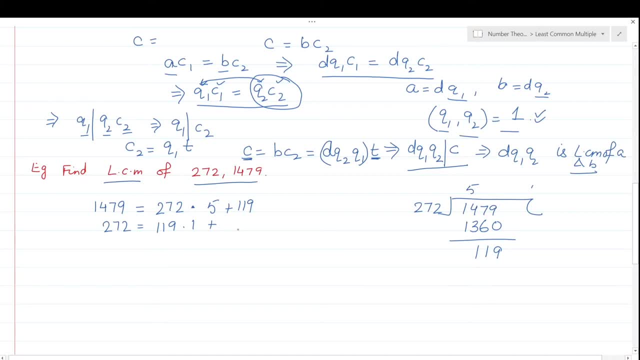 5 plus 5.. So we have 12 minus 9,, which is 3.. 6 is less. 6 minus 1 is 5.. That is 1.. So it is more than 119.. It means: 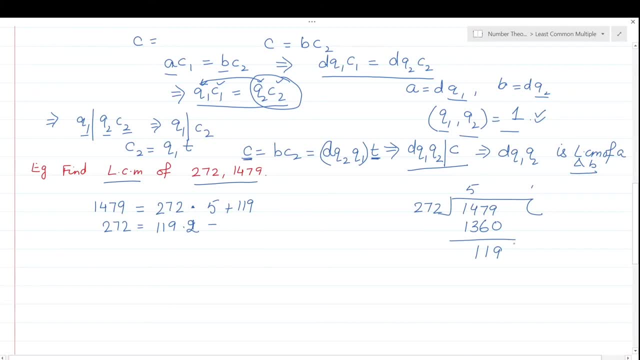 we will have to check on 2 instead of 1.. So we divide this: 272: 1, 2, 1 is 2, 2 plus 1 is 3 and this is 2.. What is left, 8 out of 12, is 4.. 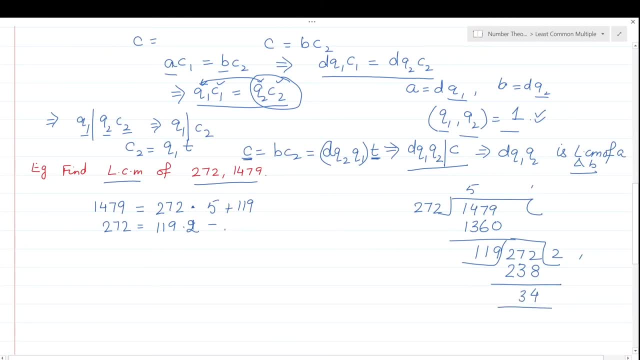 3 out of 6 is 3.. So your remainder is 34.. So we can write it as this value: This is 34.. Now we will divide 119 by 34.. So what will be the value now? 33 is 9, 3 plus 12.. 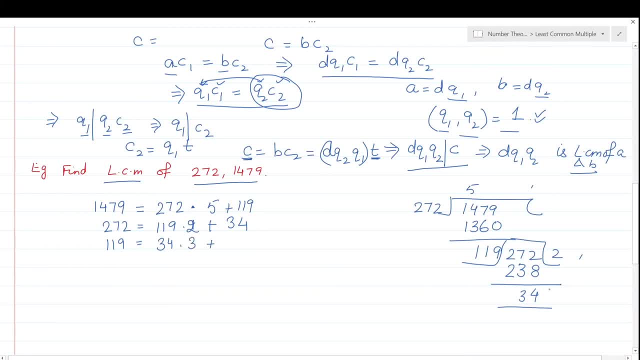 So it means it will go from 3.. What will be left? So we have to divide this number by 34 into 3. It is 4 through the 12, 1, 9 plus 1 is 10.. So it is 7 and 1.. 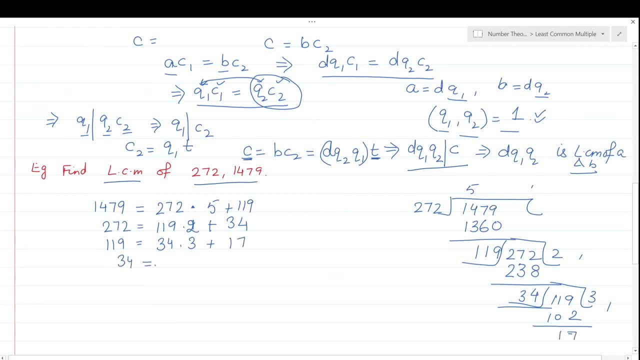 So we are left with only 17.. Now we will divide 34 by 17 into 2 plus 0. It means 17 will be your GCT. Now to find out the LCM, This is 272 into 14.. 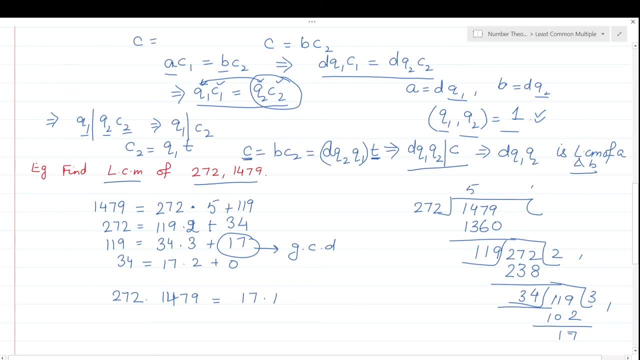 79 is equals to GCD into LCM. You have to find out. Suppose that value is L And now you just calculate this value yourself. I am not going to calculate it. Divide it by 17 and then multiply it and solve it. 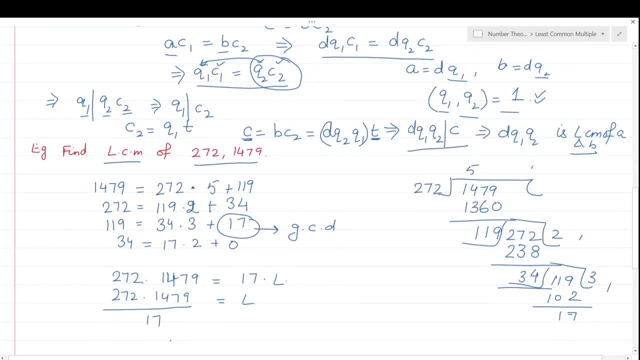 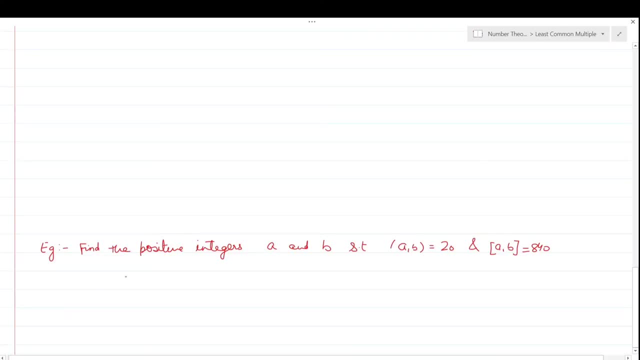 Finally, you will get your LCM. In this way, you can find out the LCM Clear Now. next we are going to prove that we have to find out two positive integers, A and B, such that their GCD is 20 and LCM is 840.. 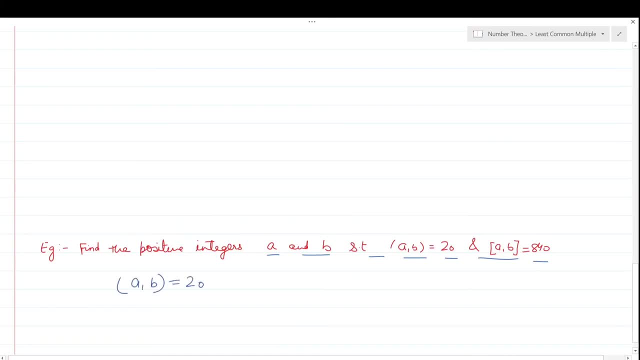 So A and B's GCD is 20.. What does this mean? We have to find out positive integers A and B such that the numbers whose GCD is 20 and LCM is 840.. So if 20 is GCD, it means 20 divides A and 20 divides B. 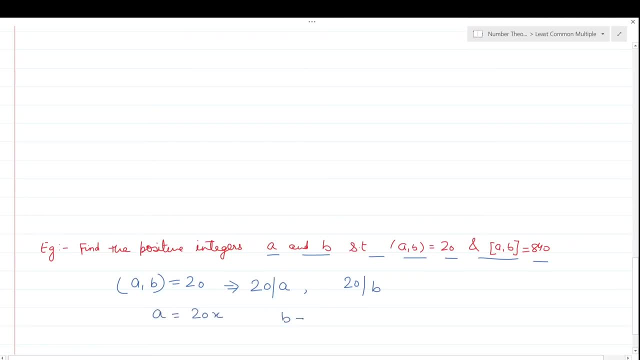 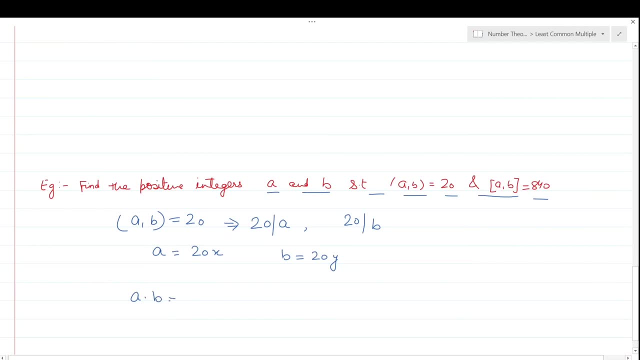 So I can write A as 20 into some number and B also as 20 into some other number Right Now, what we have done right now, Product of the numbers is equals to product of their LCM and GCD. LCM and GCD. 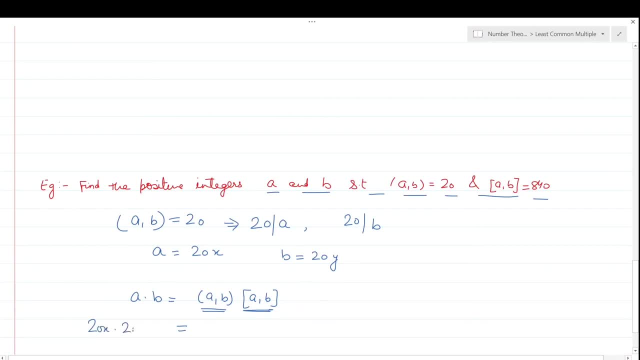 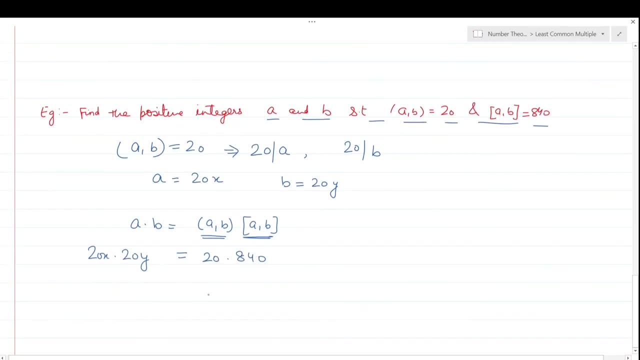 So it means A is what 20X, B is what 20Y, GCD is 20 and LCM is 840.. It means this condition will hold Now 20, cancel out. So X into Y is equals to 840 divided by 20.. 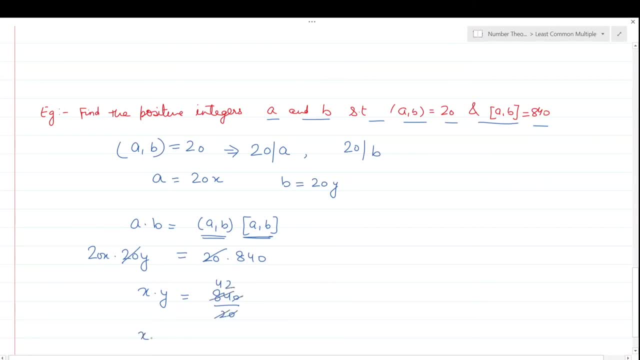 This cancels out. How much is left? 42.. So now we have to find out the values of X and Y, whose product is equal to 42. So what are the possibilities of X and Y, such that X into Y is equal to 42.? 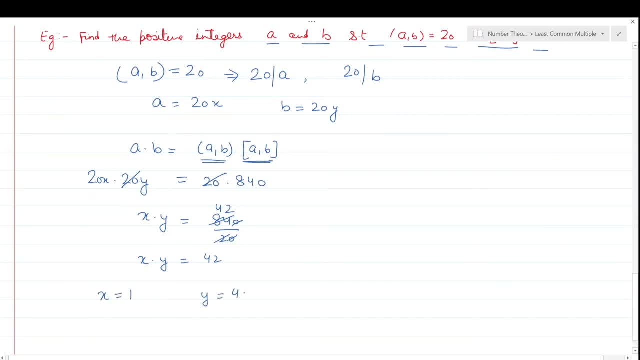 If I take X as 1, then Y will be 42. In this case, how much will be A? A was 20X, So it means A will be 20 and B will be 20 into 42.. I am substituting the values of Y. 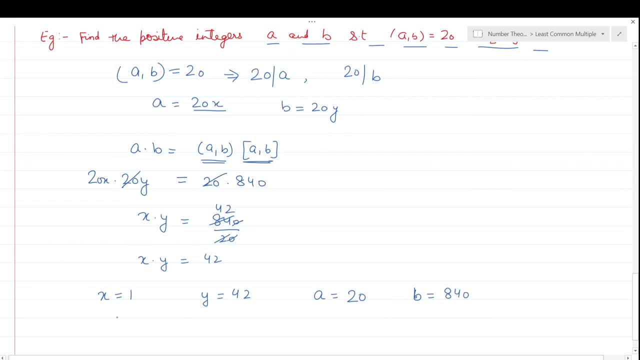 If I take X as 1,, then how much will be A 840.. Right Now, next case: what are the possibilities of X? If X and Y are the divisors of 42, then what can we take X as? 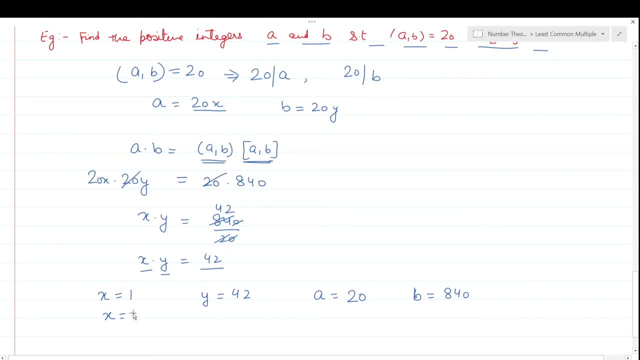 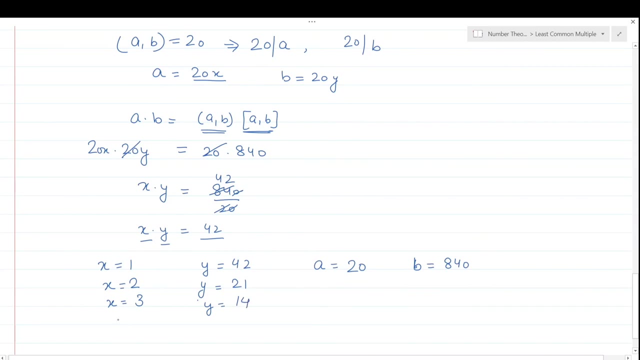 And if X is 2, then Y will be 21.. First let's check the choices of X and Y. If X is 3, then Y will be 14.. So that's it Right, 14. 14.. 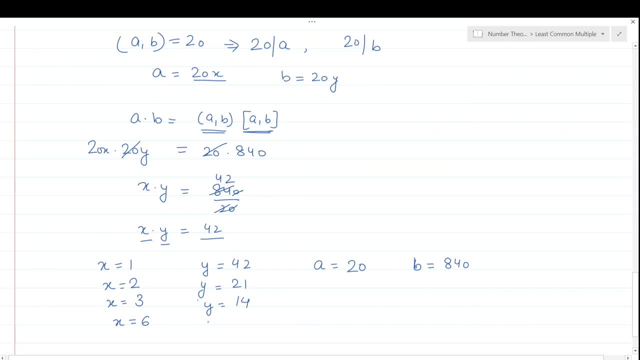 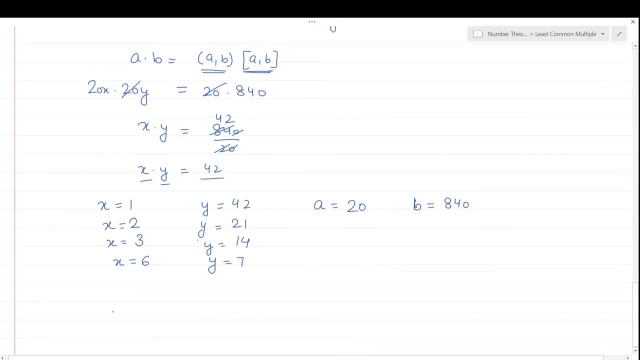 Can there be any other possibility? Yes, you can say that we can take X as 7, then Y will be 6.. So accordingly, if we reverse these numbers, X will be 14, Y will be 3.. In that case, A and B will be interchanged. 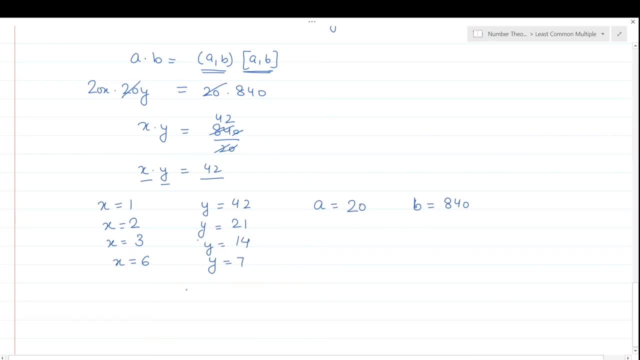 But the numbers will be the same. That means the same set of numbers will come, which X is 1,, 2,, 3,, 6, and Y is not the corresponding values. If we take Y as 1,, then Y will be 3..